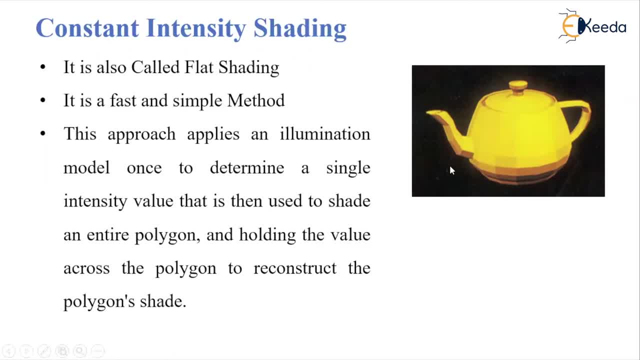 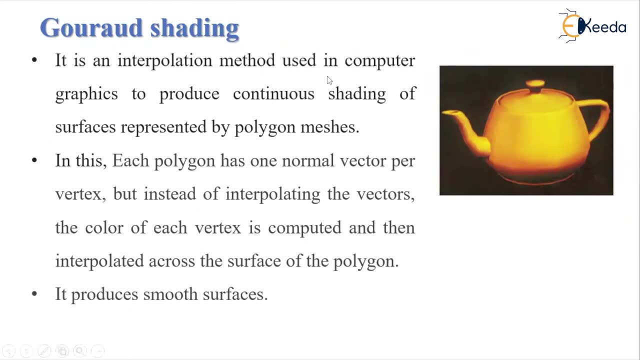 So this method is quite accurate, But it can be more accurate by introducing the other methods. Okay, So we will see the next one, that is, the Gorod Shading. It is an interpolation method used in a computer graphics to produce continuous shedding of the surfaces. 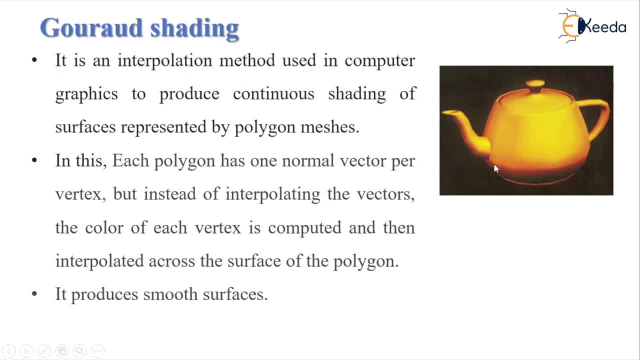 represented by the polygon mesh. So it is represented with the help of polygon mesh and it gives us more accuracy than the flat shading. In this each polygon has one normal vector per vertex. So, as we have seen, the polygon is have different vertices, So per vertices there is one normal vector is used. 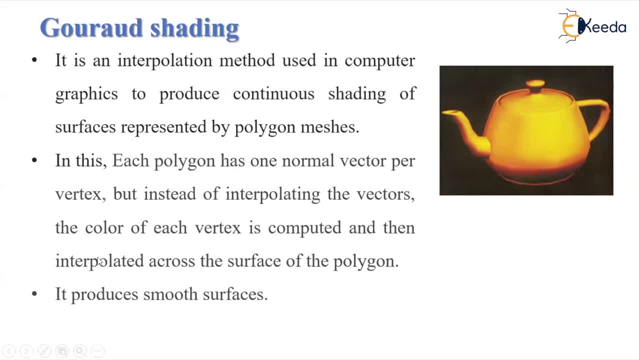 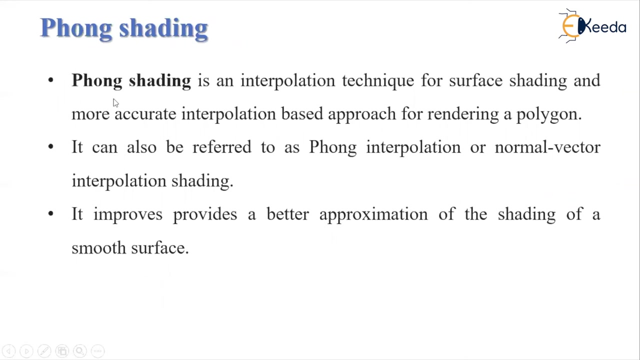 but instead of interpolating the vectors, the color of each vertex is computed and then they interpolated across the surface of the polygon, So it produces a smooth surfaces compared to the flat shading. Now next is the form shading. This is this. one is the more accurate shading. 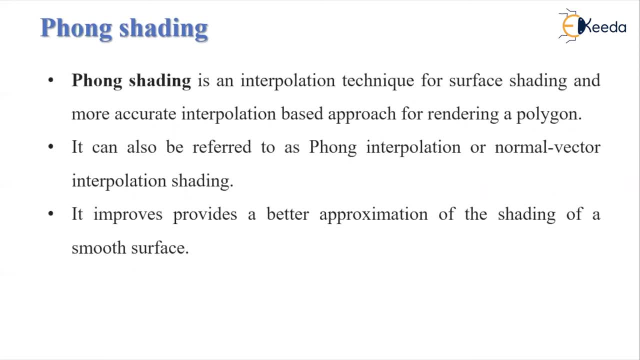 technique than the previous two. So it is an interpolation technique for surface shading and more accurate interpolation based approach for rendering a polygon. It can also be referred to as form interpolation or normal vector interpolation shading. Now form is nothing but the name of the scientist, like a Goddard. It improves, provides a better 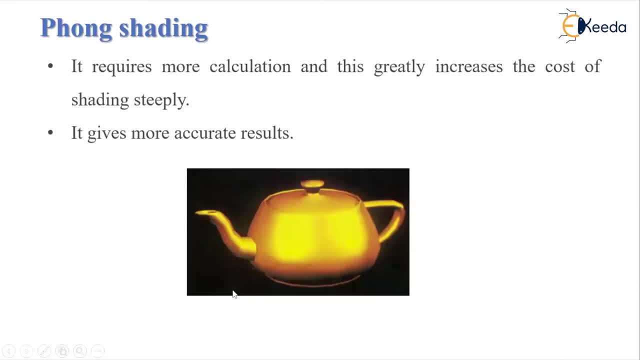 approximation of the shading of a smooth surface, So it requires more calculation. as we have seen, it is more smooth than comparative to flat shading and Goddard shading, So that's why it needs to be more accurate. It needs more calculation and it this greatly increases the cost of shading. 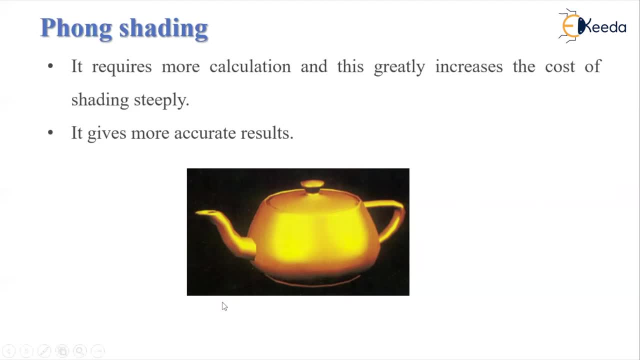 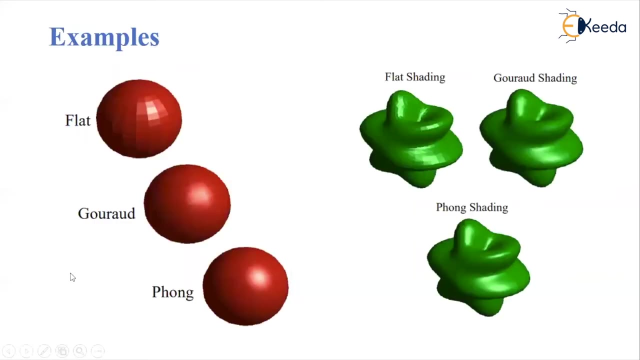 splitly. So the cost. it is quite expensive and it is complex to build such objects. It is quite complex to design such object with the help of form shading, but it gives you the more accurate result compared to other two. So see, these are the certain examples of the three different types of